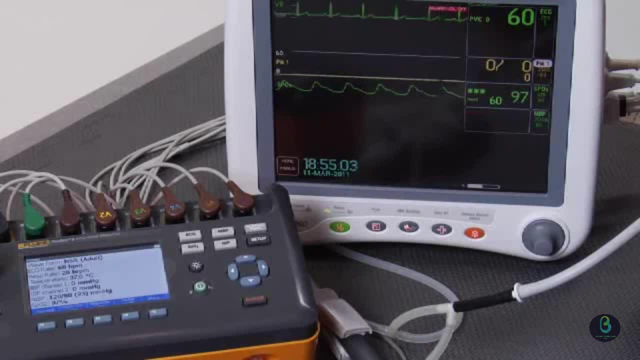 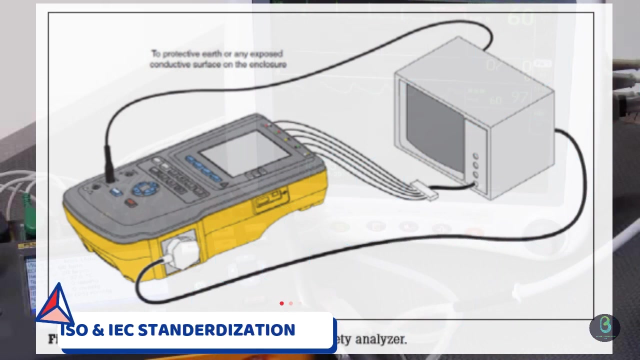 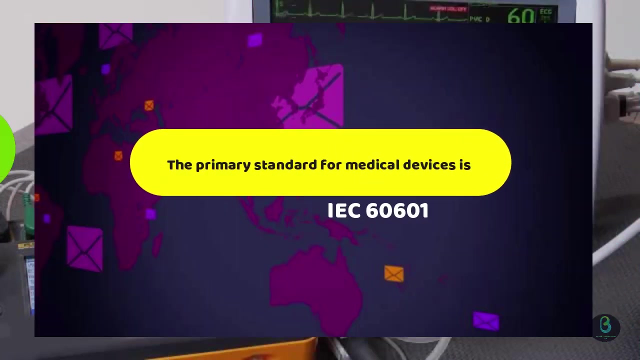 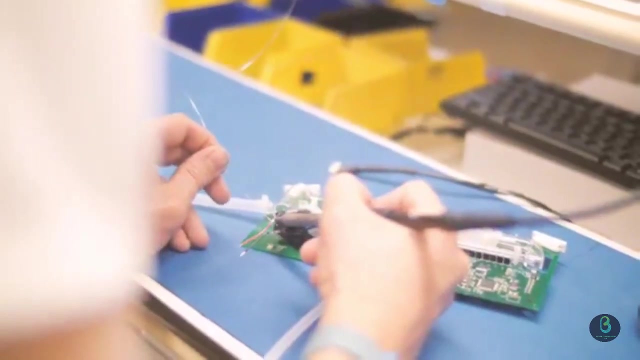 in partnership with a world trade organization. These include standards for electro-medical equipment. There are general and specific standards for medical device electrical safety. The primary standard for medical devices is IEC 60601.. General requirements for protection against electric shock hazards are covered in IEC 6060.. 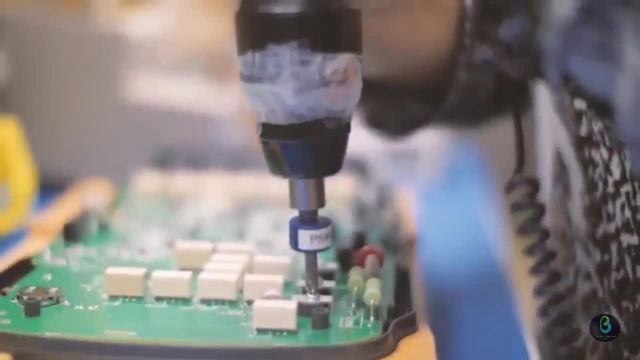 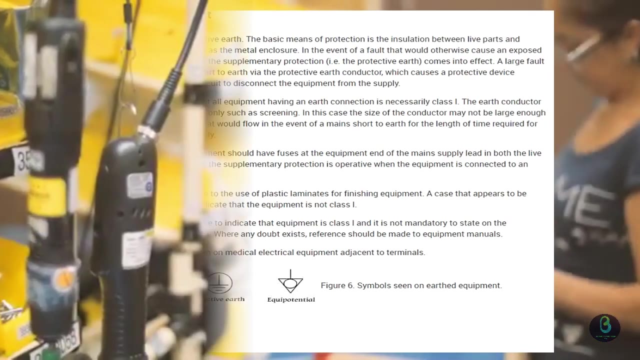 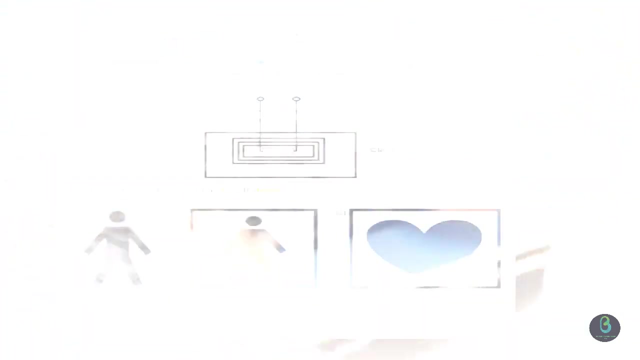 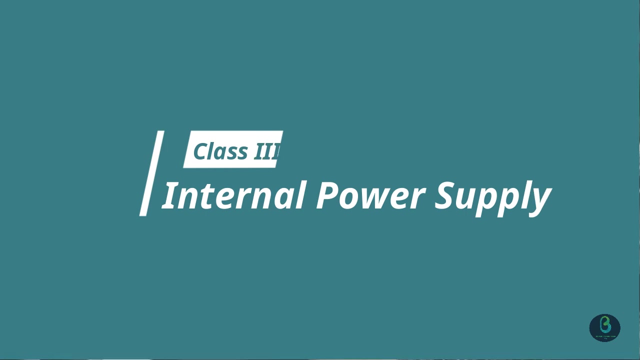 First, in this standard each instrument has a class Class 1 Live part covered by basic insulation and protective earth. Class 2 Live part covered by double or reinforced insulation. Class IP- Internal power supply. Second, each patient applied part or patient lead has a type. 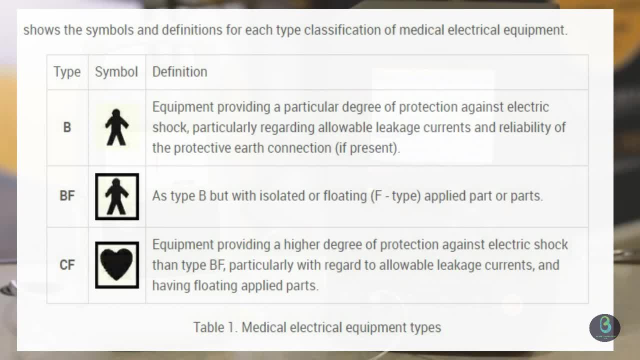 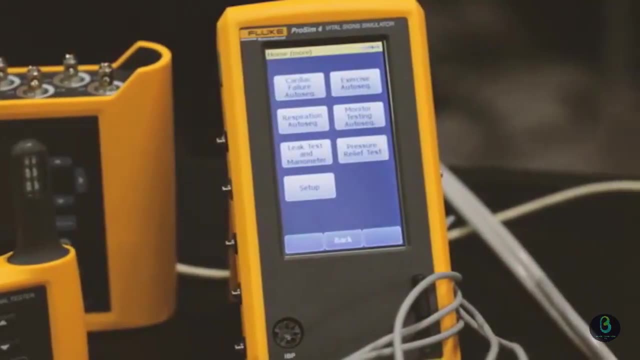 Type B- Patient applied part earthed. Type BF Patient applied Part floating surface conductor. Type Cf. Type Cf- Patient applied part floating for use in direct contact with a heart. Type Cf- And leakage measurement limits have been developed for equipment types and measurements. 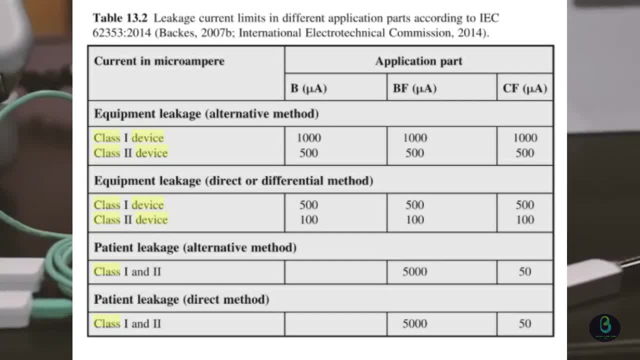 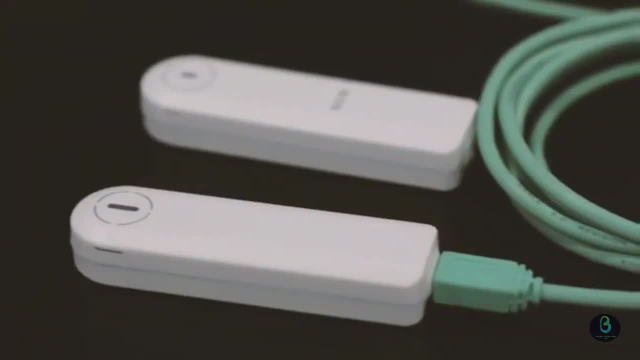 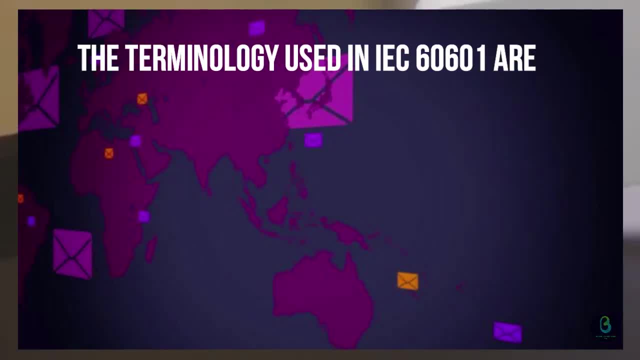 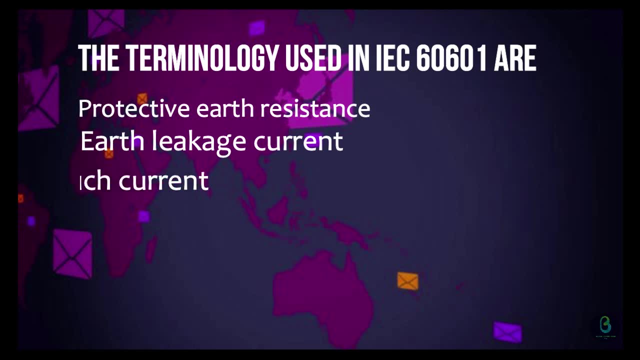 Type Cf, Type Cf, Type Cf, Type C, Type Cf, Type Cf F. actor gas discharge, Daison, high temperature, small heart type. Type E, Type E, Type it, Type C, Type C, Type N, Type C, Type I, Type S, Type K, Type L. 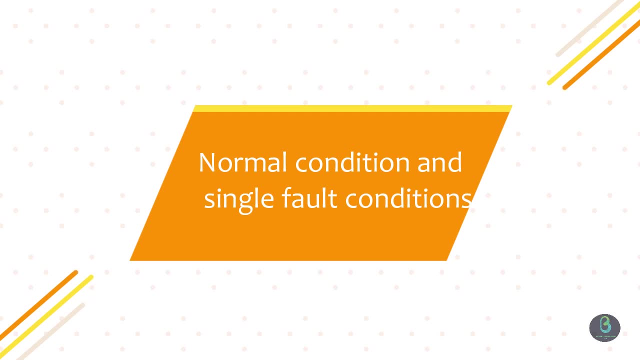 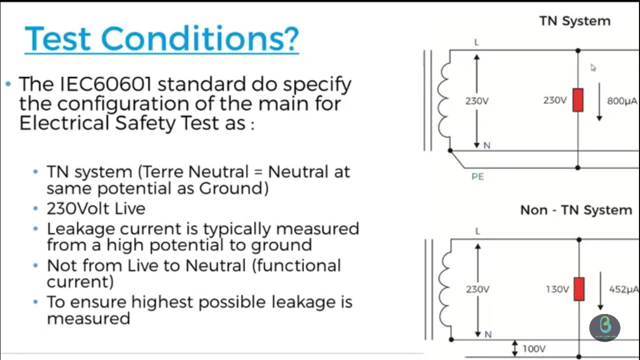 Type Z, Type V, Type A, Type Z- Single Fault Conditions. A basic principle behind the philosophy of electrical safety is that in the event of a single abnormal external condition arising or the failure of a single means of protection against a hazard, no safety hazard should arise. 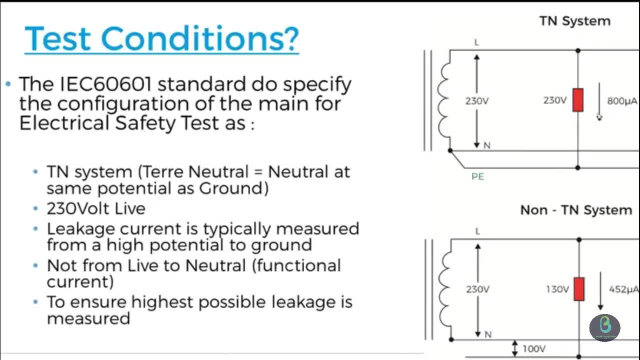 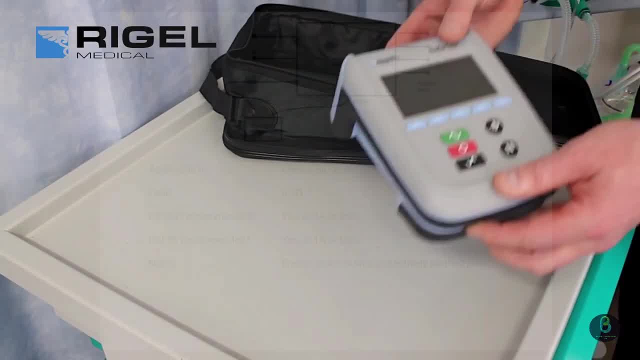 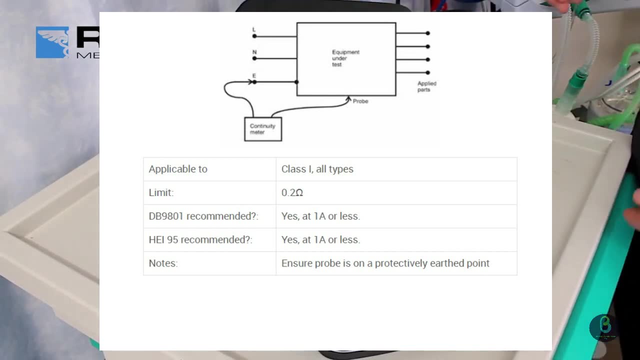 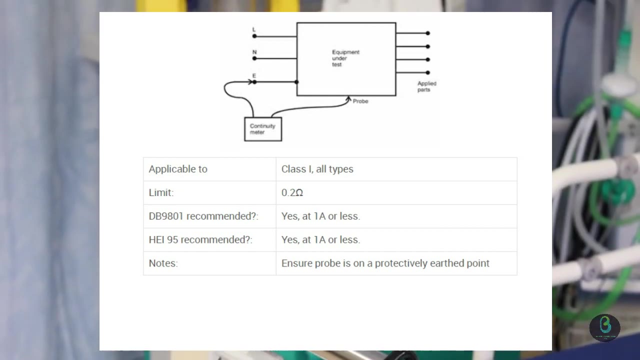 Such conditions are called single fault conditions. Protective Earth Continuity. The resistance of the protective earth conductor is measured between the earth pin on the mains plug and a protectively earth point on the equipment enclosure. The reading should not normally exceed 0.2 ohms at any such point. 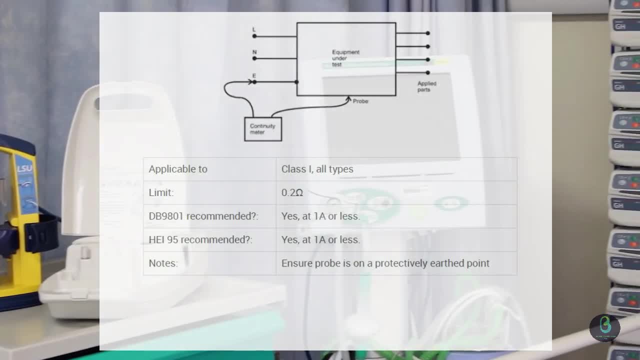 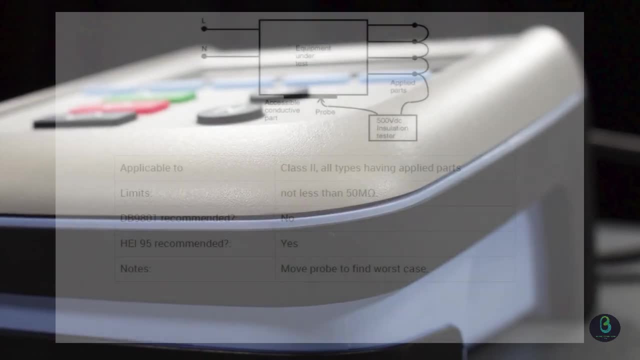 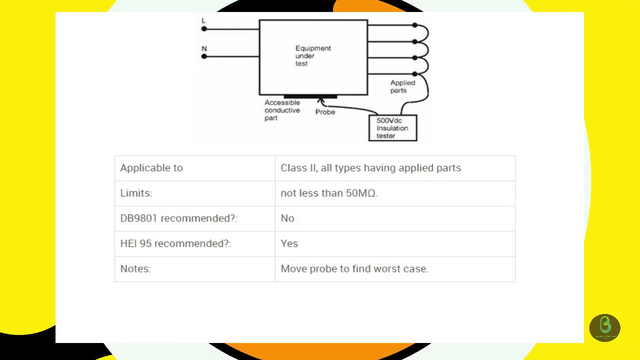 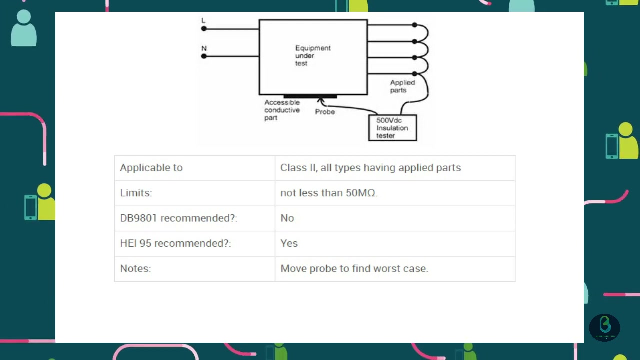 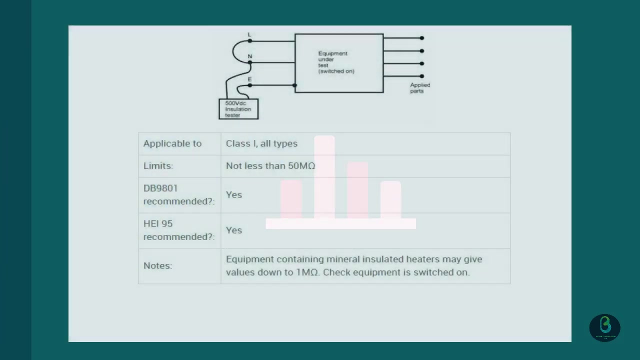 The test is obviously only applicable to Class 1 equipment Insulation Tests. IEC 60601 1 lays down specifications for electrical separation of parts of medical electrical equipment, compliance to which it is essentially verified by inspection and measurement of leakage currents. Further tests on insulations are detailed under dielectric strength. 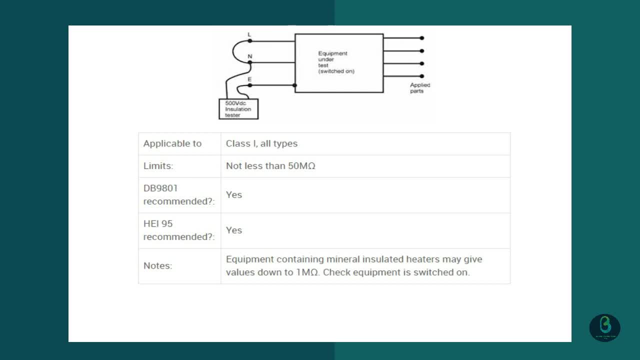 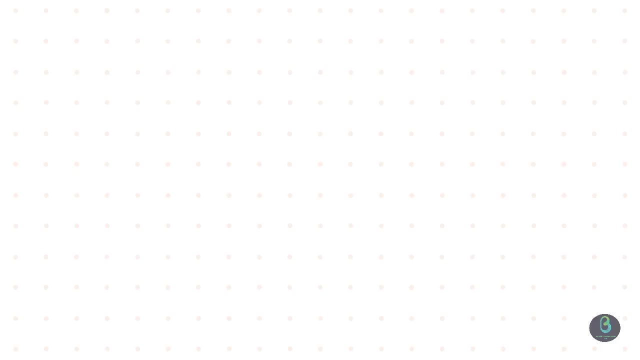 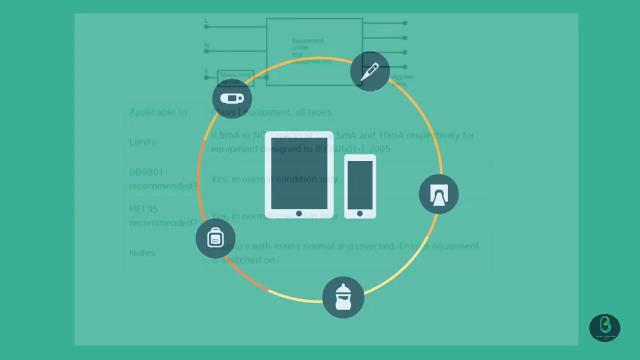 These tests use AC sources to test equipment that has been preconditioned to specified levels of humidity. The tests described in the standard IEC 60601 are not necessarily effective in the case of an electric circuit with the use of a partial-dipole. 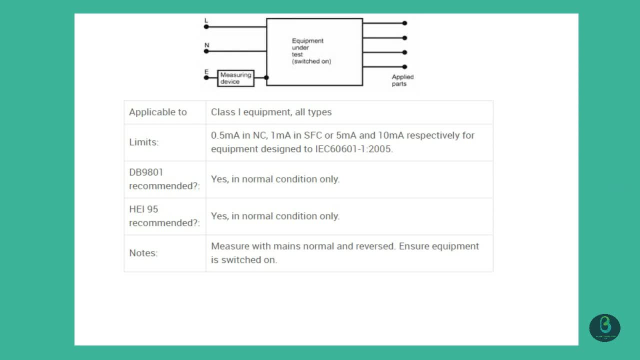 of 99.86 kohm. The pressure of the standard IEC 60601 is normally around 0.65 ohms against the teeth. The temperature of the IEC 60601 can beically measured at any time. In any case, the current must be measured as shown in Figure 12.. 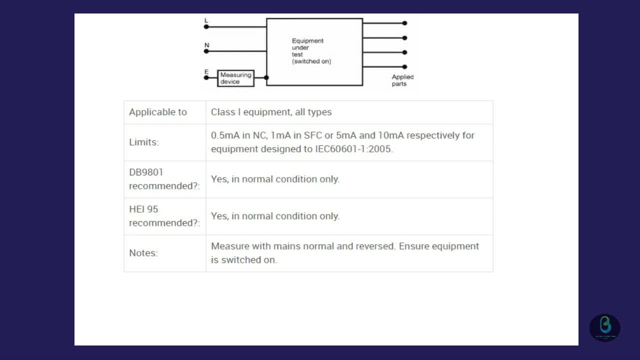 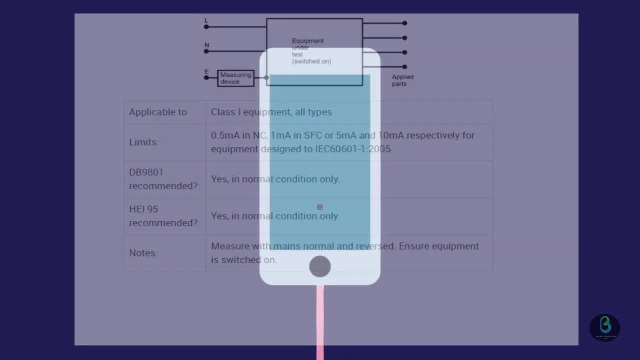 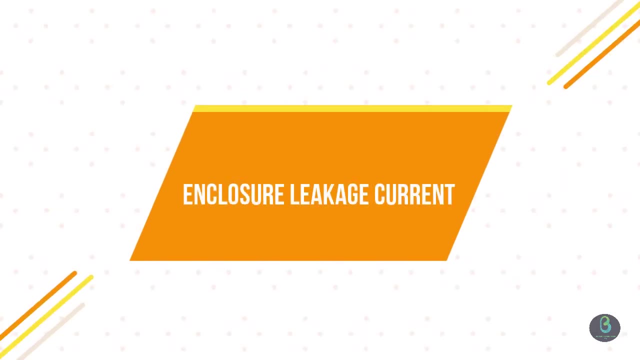 The current should be measured with the mains polarity normal and recommended that the earth testers offer the opportunity to perform the test under single-fault condition. This arrangement normally gives a higher leakage current reading. Enclosure: leakage current is measured between an exposed part of the equipment which is 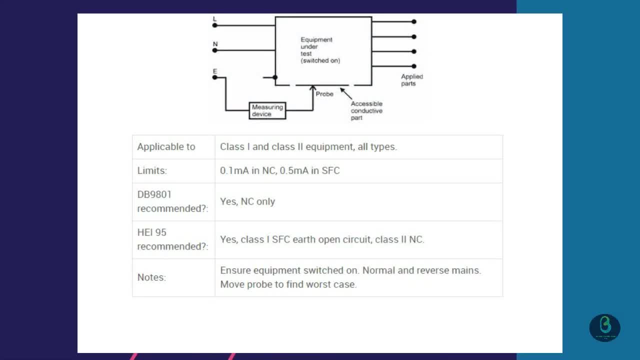 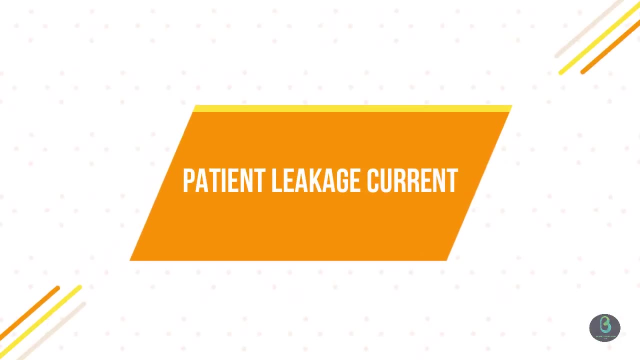 not intended to be protectively earthed and true earth. The test is applicable to both Class I and Class II equipment and should be performed with mains polarity, both normal and reversed. Patient Leakage Current For Class I and Class II, Type B and BF equipment.